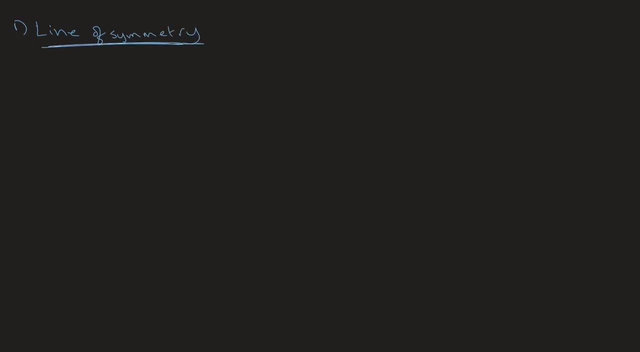 I'll explain to you what this is using a visual example. So in any given, In any given quadratic equation- let's say this one or this one, I'm not going to assign any values to it- there's a line of symmetry which runs down the center. 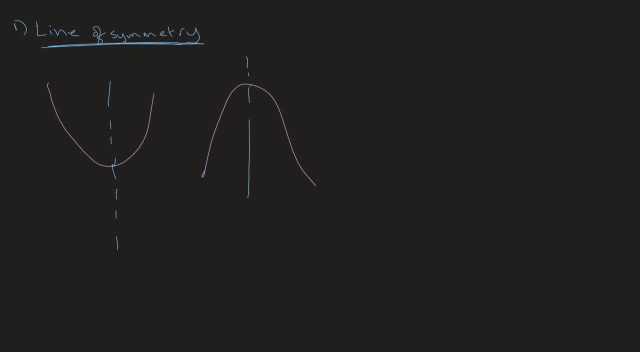 And what that essentially means is that our graph or our quadratic equation can be reflected inside of the line of symmetry. So that means that the distance from here to this point is the same as the distance from here to the corresponding point. So that's the line of symmetry. 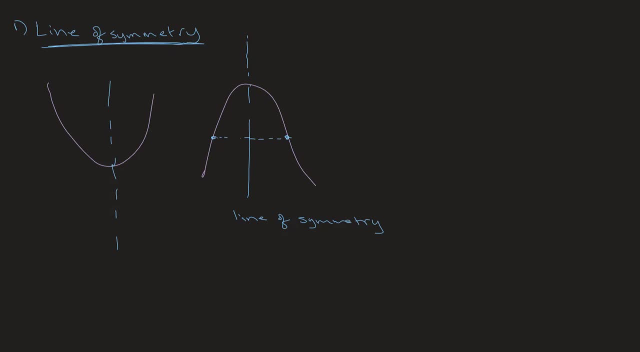 And using or finding the line of symmetry proves to be very useful when we're solving for maximum or minimum points, because they always run through the maximum or minimum point of our curve. So let's look at an example of a question for which we have to solve for either the 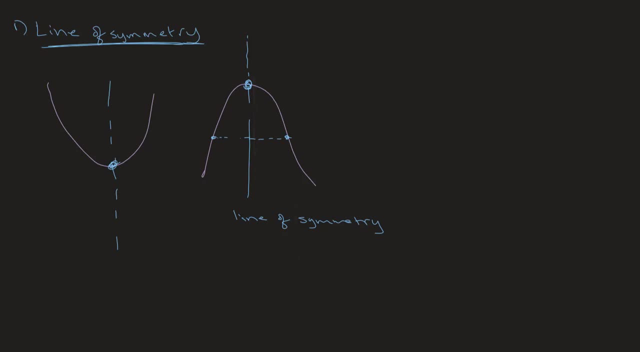 maximum or minimum point. So let's say that we have- Let me scroll down here- X squared Plus 4x Minus 5. And we have to find either the maximum or minimum point. Well, straight off the bat we can tell that it's going to have a minimum point. 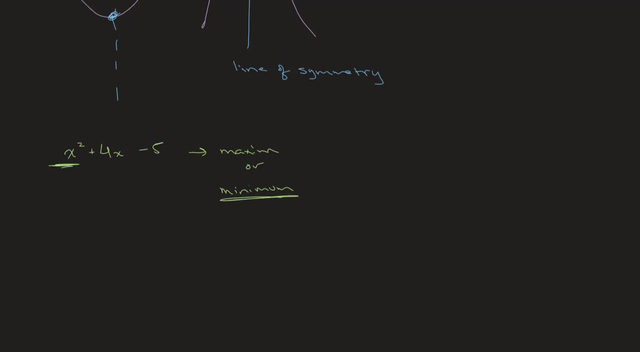 And that's because the coefficient of x squared is 1, which is greater than 0. So we know that we're solving for a minimum point. Now for this question, I'm just going to draw out the graph so that we have a. 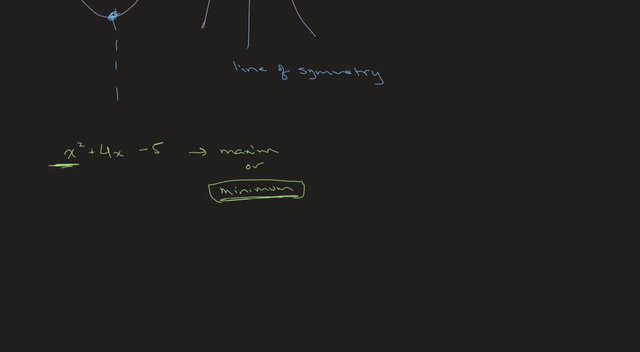 So you have an idea of what we're trying to solve for over here. So we have our axes- this is our y-axis and this is our x-axis- And then we have our graph, which looks something like this, going up on both sides: 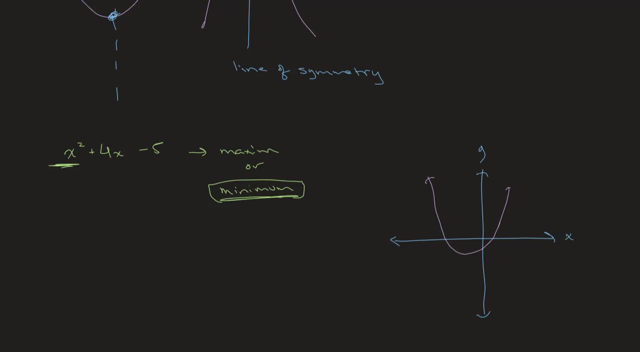 Now the way that we solve for the line of symmetry is we find two points on the curve with the same y-value, So in this case we'd be looking at the point of intersection along the X-axis, So where the y-value is 0.. 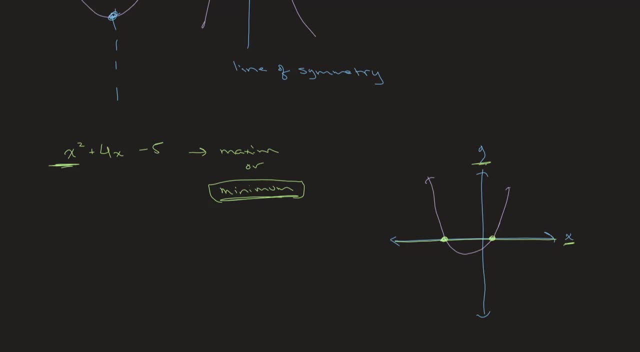 So we'd be trying to solve for these two points And the line of symmetry which looks something like this, would be right in between them. So at our intercepts, y is equal to 0.. Which is equal to x squared plus 4x. 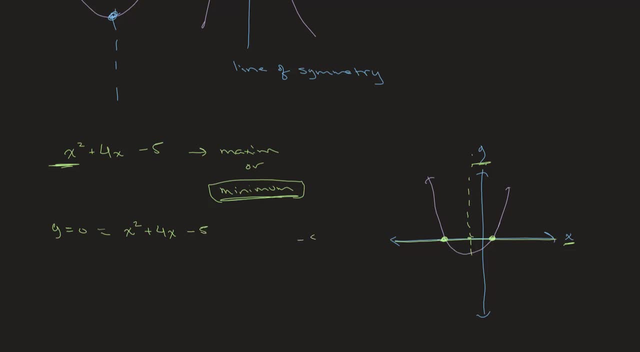 Minus 5.. We have minus 5 over here. We can use minus 1 and 5.. So x squared Minus x plus 5x minus 5 is equal to 0.. X times x minus 1 plus 5 times x minus 1 is equal to 0.. 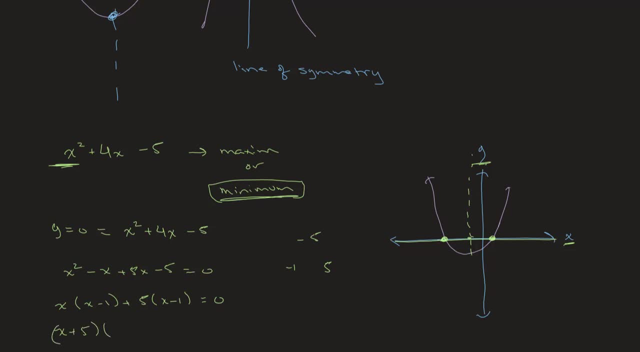 X plus 5 times x minus 1 is equal to 0.. From this we get two possible values of x. We get: x is either equal to negative 5 or x is equal to 1.. And in both cases y is equal to 0.. 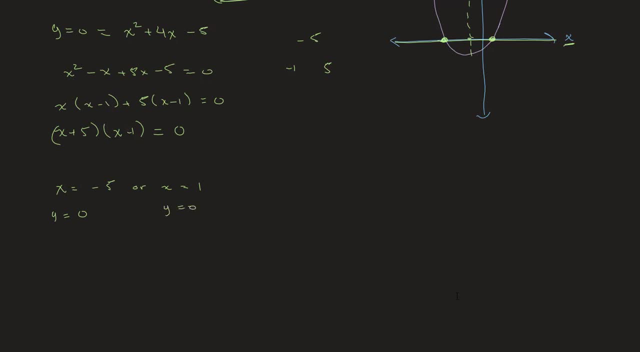 So we get x squared plus 4x minus 1.. And in both cases y is equal to 0.. And in both cases y is equal to 0. So let's mark that up on our graph. Here we have the value of 1.. 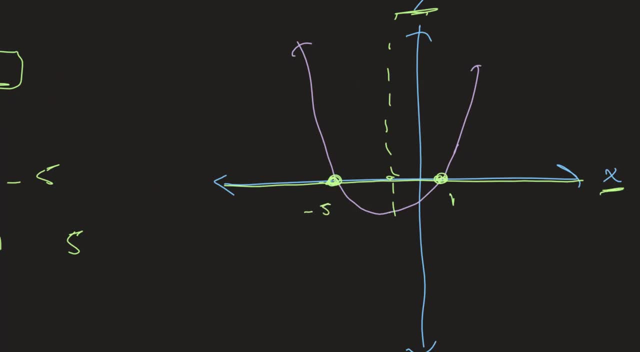 And here we have the value of negative 5.. Now, as I mentioned earlier, the line of symmetry runs directly in between these two points. So the distance from, say, here to here will be the same as the distance from here to here. 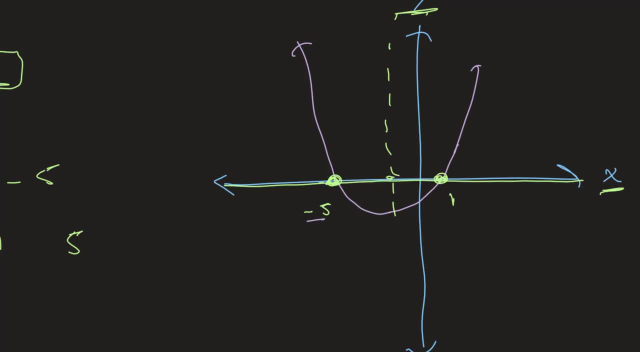 So right off the bat we can tell that minus 5 and 1 are six points apart, because this here is five units and then this right here is one more unit. So they're six units apart. That means that the point in between them 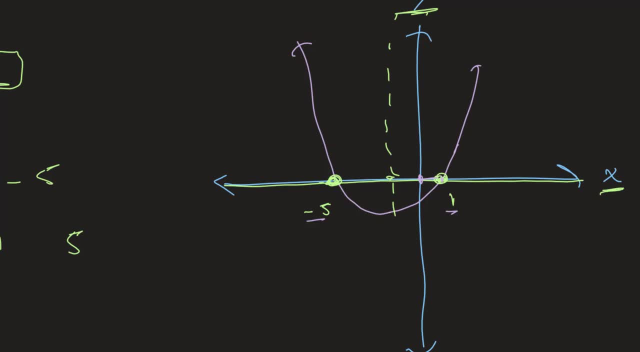 is three units apart from both of them. So they're six units apart and the point in between them is three units apart from both of them. So three units away from negative 5 is right here, negative 2.. And three units away from negative 1 is also. 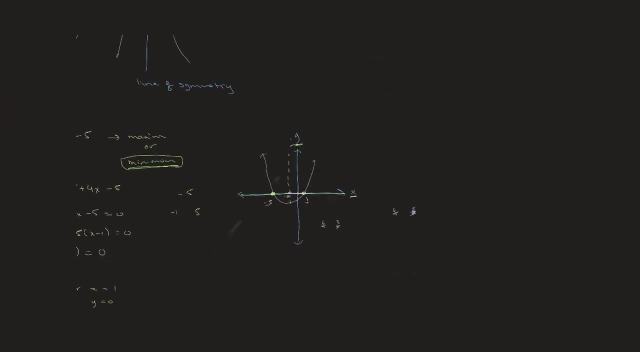 negative 2.. So we know that our line of symmetry runs through, or it actually is. the line x is equal to negative 2.. So, as you can see, there is a line that's already made. running through the point x is equal to negative 2.. 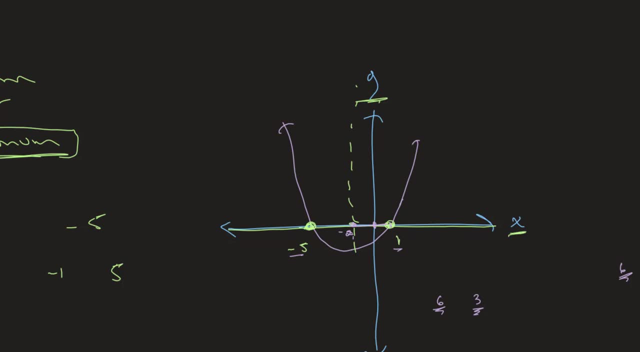 And, as I mentioned earlier, we also know that the minimum point is touching this value or this line of symmetry. So the minimum point touches the value that we have of x is equal to negative 2. So we have the x value of our minimum point. 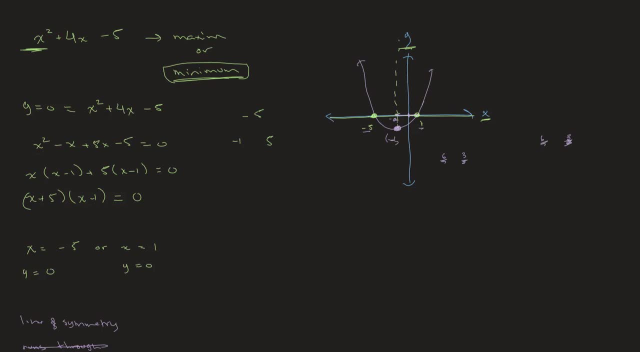 so it's minus 2 something. And to find the y value we simply plug negative 2 into our equation. So we get y is equal to negative 2.. So we get y is equal to x squared plus 4x minus 5.. 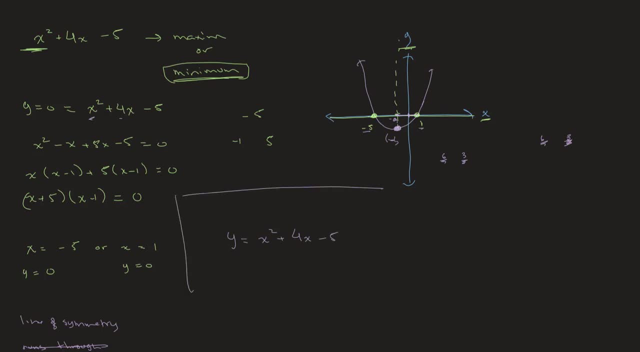 Let's box this off. So we get: y is equal to negative 2 squared plus negative 2 times 4 minus 5.. This gives us 4 minus 8 minus 5, which gives us a value of negative 9.. So the y value of our minimum point is negative 9.. 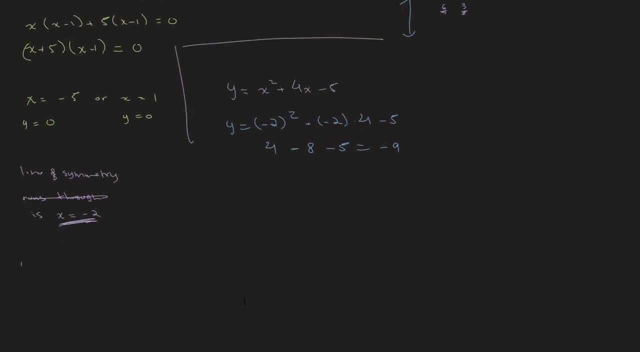 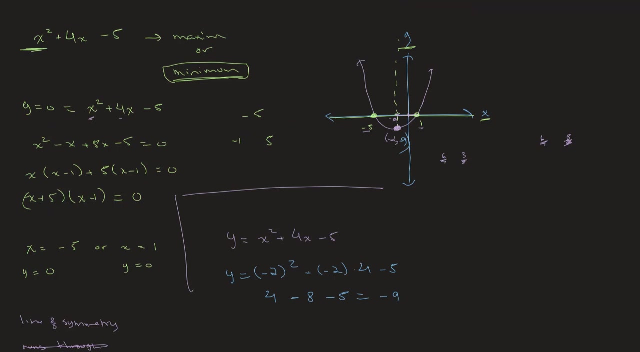 So write this out. This is our final answer. The minimum point of our curve is at the point minus 2 minus 9.. So, just in review, what we did was we found the line of symmetry using our points of intersection, And using that we found the minimum point of our curve. 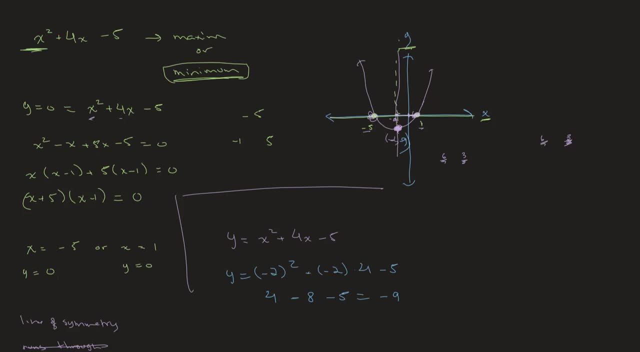 because we know that the minimum point runs through, or the line of symmetry runs through the minimum point. So that's the minimum point of our curve. Now the second method, which I mentioned before and, as I said, I won't be going into much depth about. 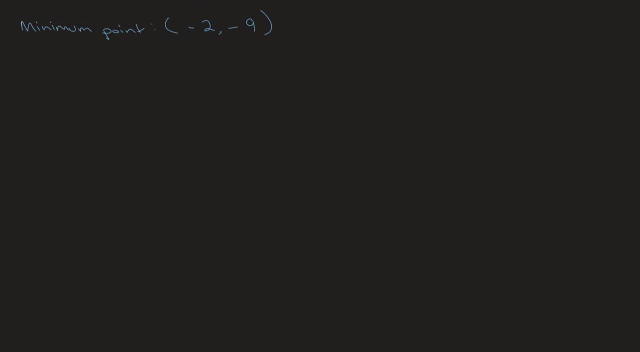 of solving for the maximum or minimum point is by completing the square. So, by completing the square, Now, what that is is essentially, we have our equation, ax squared plus bx plus c, And we rewrite it using methods that I'll explain in my next video. 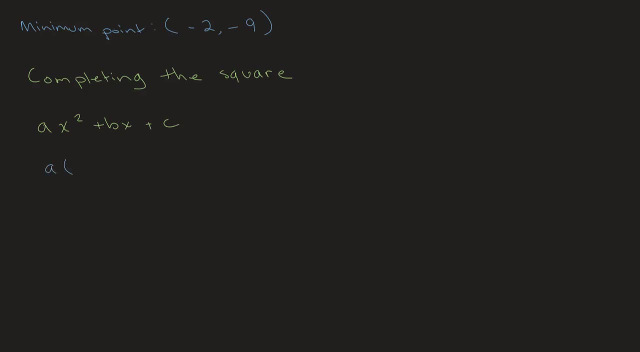 in the form of a times x minus h whole squared plus k. So we originally had this equation of ours And from that we got a times x minus h squared plus k, And from this we get the minimum point, or we get the minimum or maximum point as h.